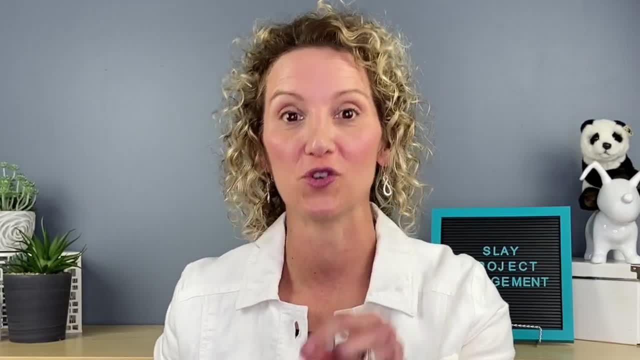 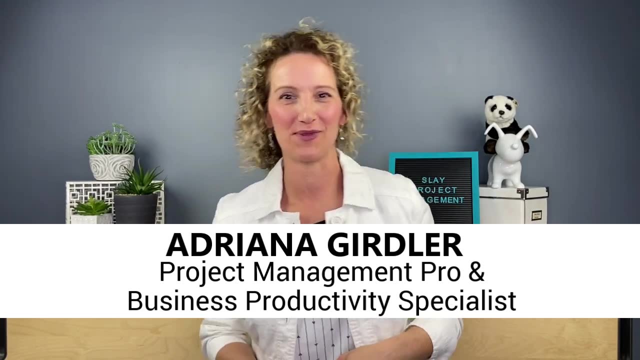 to the end of this video because I have something for you that's going to be really cool to ensure that you're successful when you're planning it out. Hi, if you're new here, welcome. For the best career and project management advice, please subscribe to my channel. hit that bell button. 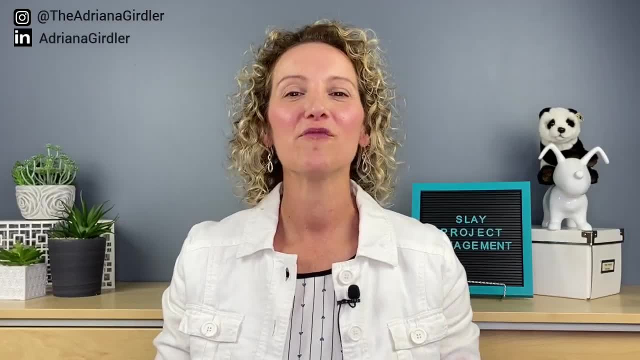 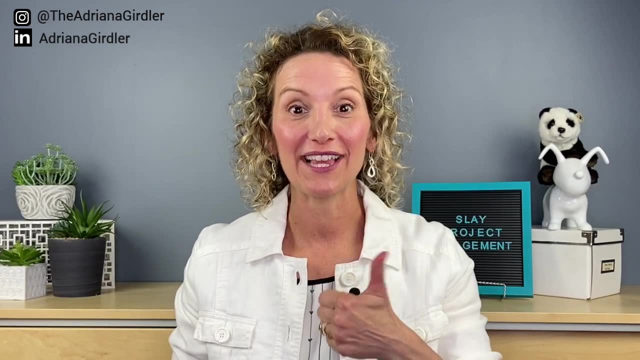 and a new video is going to come to you every Wednesday. I've planned tons of projects in this exact way that I'm about to share with you, So if you're excited, as I am, give this video a like and let's get to it. Step one, project goals and deliverables. Congratulations, you got the project. 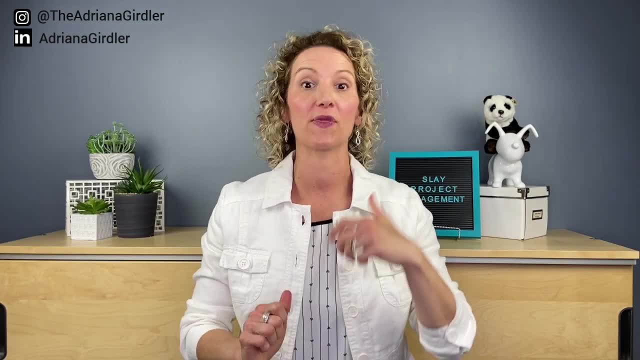 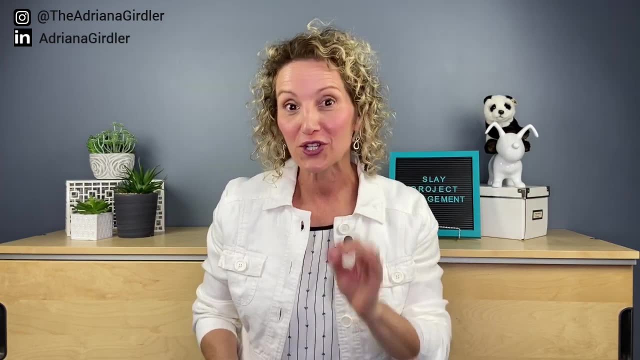 and you're probably told what it is. Now you have to have an understanding what the project goals and deliverables are, And this you get from the sponsor. This is the person who's in charge of the project. This is critical because so many times this is not clearly understood. 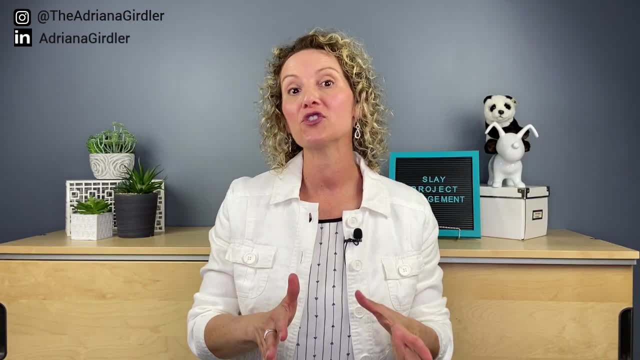 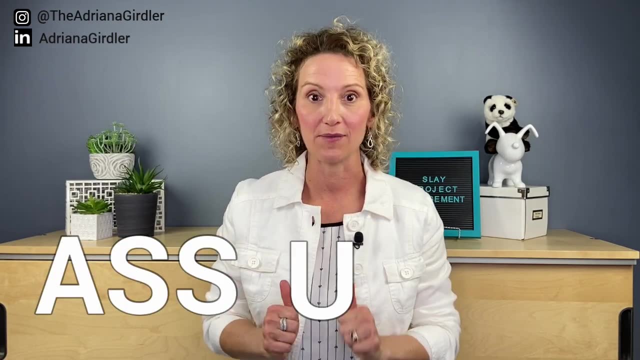 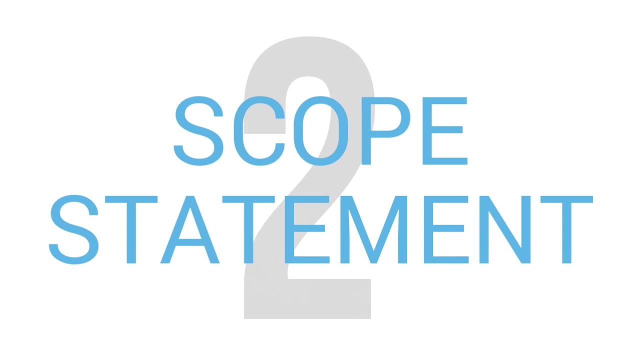 And this is how projects get in trouble: When you don't understand project goals and deliverables and you assume them. guess what? It makes an ass out of you and me, And that is not a great way that you want to be starting off your project. Step two: scope statement. All right, you want? 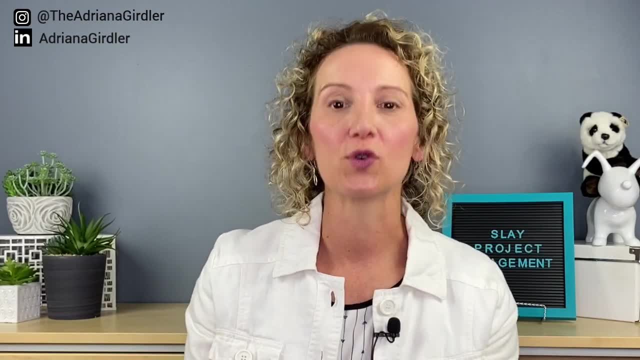 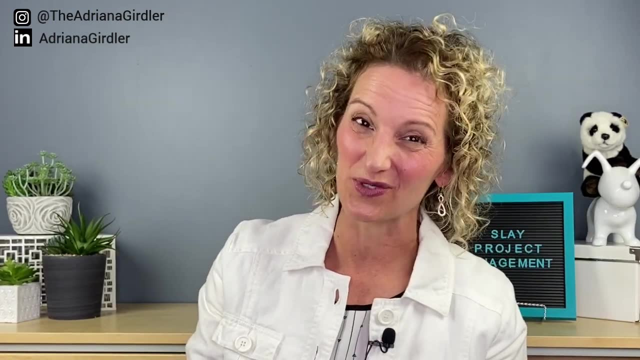 to be creating this with the project sponsor. In the ideal world, they would have given this to you and said: hey, I gave you this project. Here is a scope statement. Unfortunately, that doesn't really happen, So you need to create this. This is a very pivotal part of your project plan. 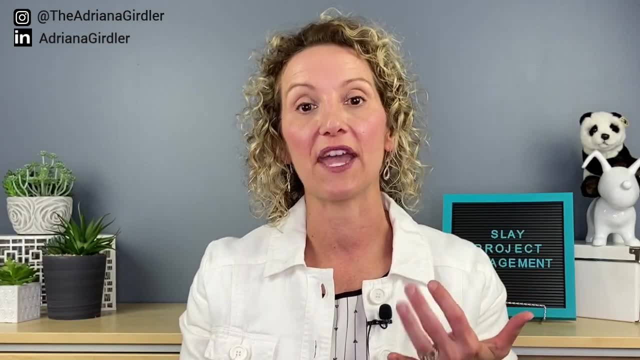 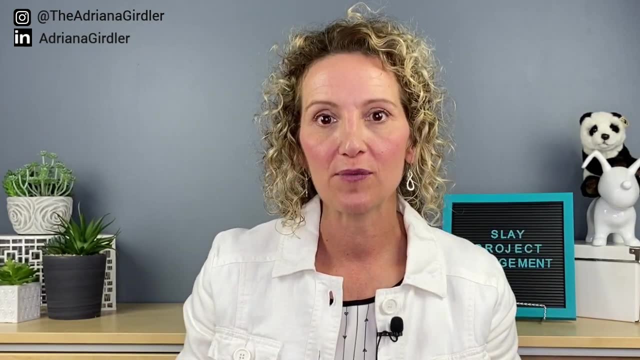 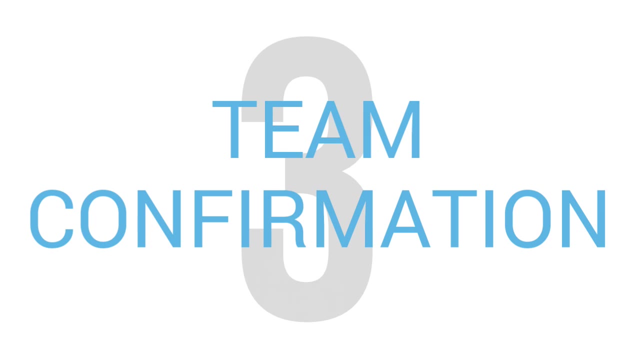 because this is going to lay out for you What exactly is it that you're delivering on, sort of the high level parameters, and by laying out what's in and out of the project, This keeps everybody on the same page And it's a very critical component of project planning. Step three: team confirmation- Find. 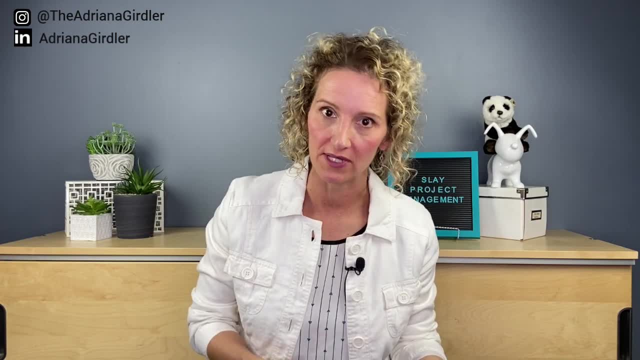 out who you need to have on your project based on scope statement. Do you see how important this is? The scope statement is going to tell you- That's a phenomenal thing. I know you are going to come in feel how going to tell you who you need to have involved. Not only that: find out if 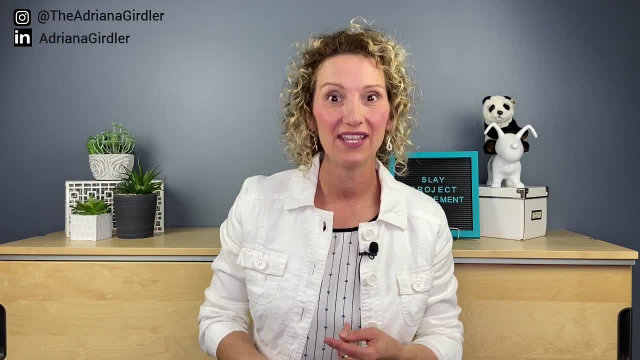 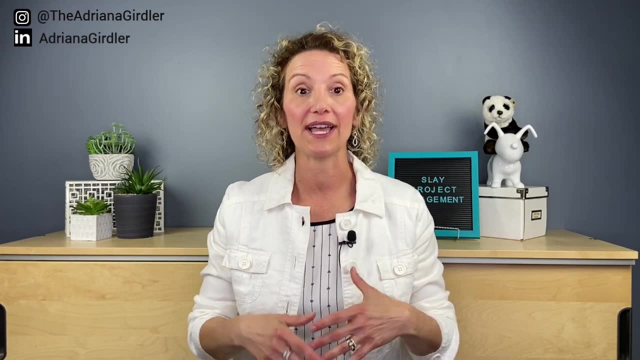 you're going to have any full-time people on the project, part-time people on the project, as well as find out how that's going to impact on the work that they're doing, because your team confirmation is critical, as your subject matter experts who are on the team are really going to help you with the. 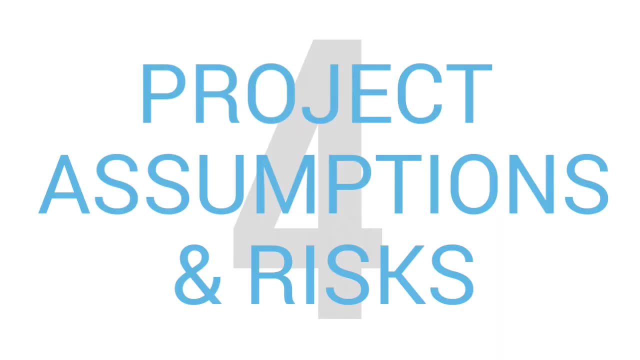 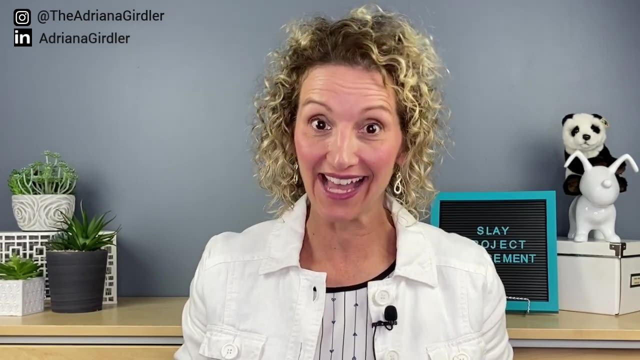 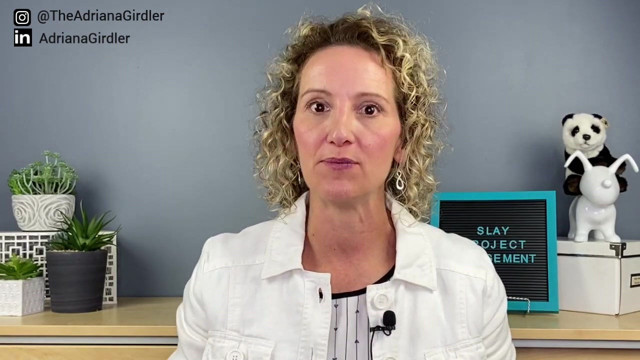 delivering of the project success. Step four: project assumptions and risks. Okay, remember what we said earlier on about assume makes an ass out of you and me. Well, this really becomes very important here. You need to reach out to key people. 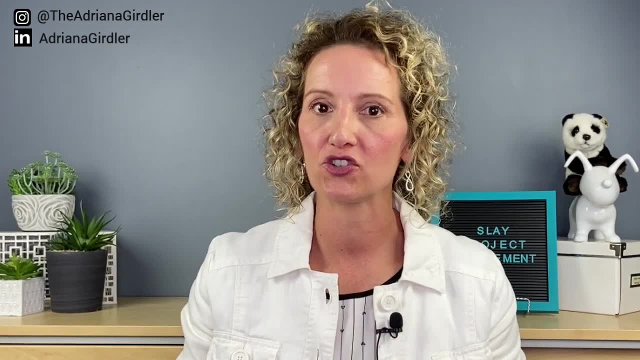 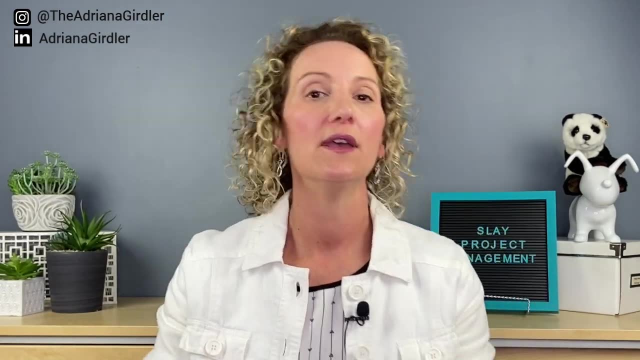 sponsors, steering committee members, your managers, subject matter experts. By the way, if you don't know the definition of all this, you can actually check out a video I have on definitions for projects. But, that all being said, you need to. 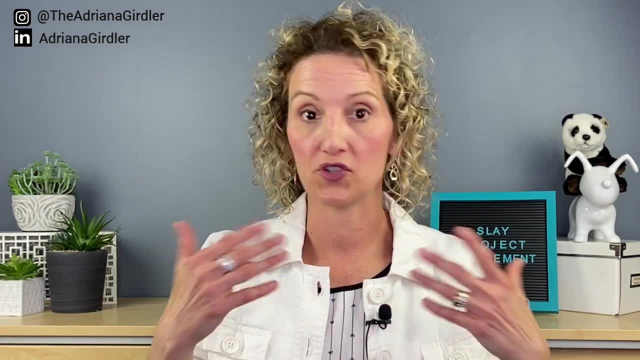 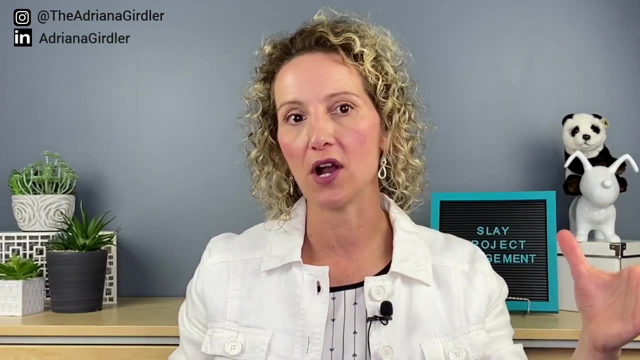 mitigate the high-level stuff. There are individuals who understand what's going on with this project and will have assumptions, And if you don't get those assumptions out, then they're going to be working off of assumptions and you're gonna have no clue what they are, and that's how you get a lot of issues. 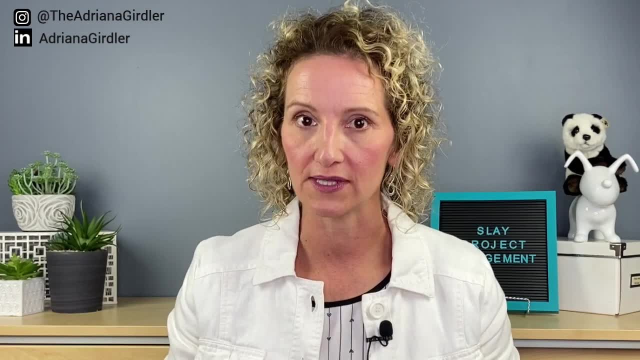 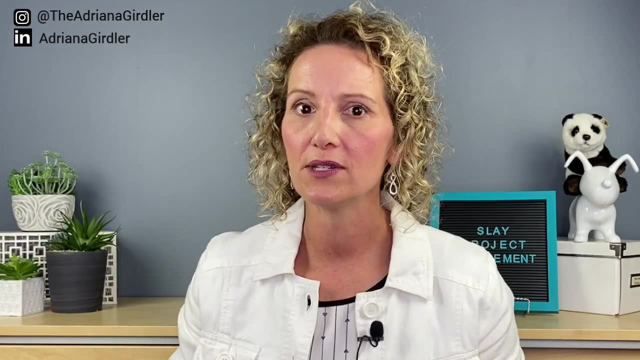 in projects. Not only that, you want to know some high-level risks. Yeah, the project hasn't started yet and there's gonna be new risks that come about when you start executing stuff. but you probably know some very high-level risks and they may not even be project related. They could be organizationally related. 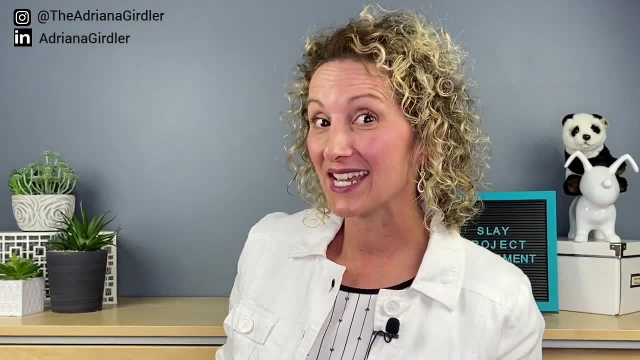 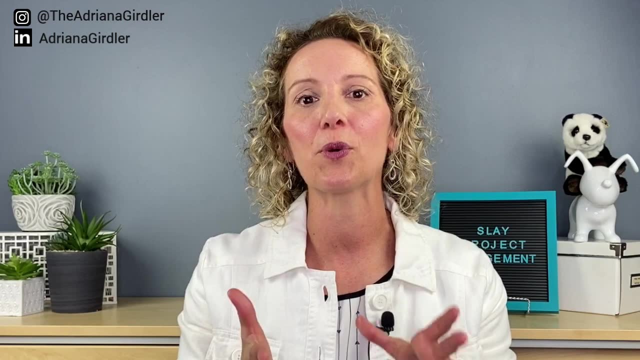 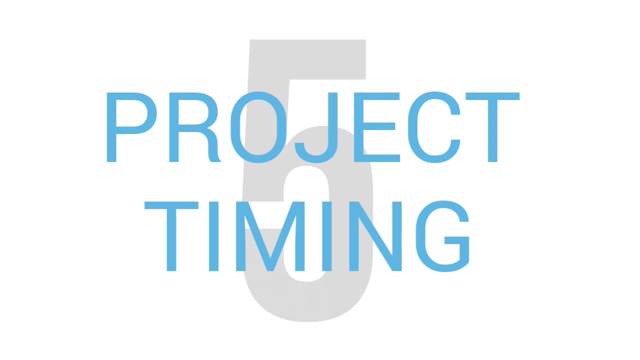 but will impact your project like nine times out of ten. that's usually resourcing. Do you actually get the resourcing that you need? So you've got to know what's in place and it's important that you at least touch upon them in the beginning of your project planning. Step five: project timing. Okay, 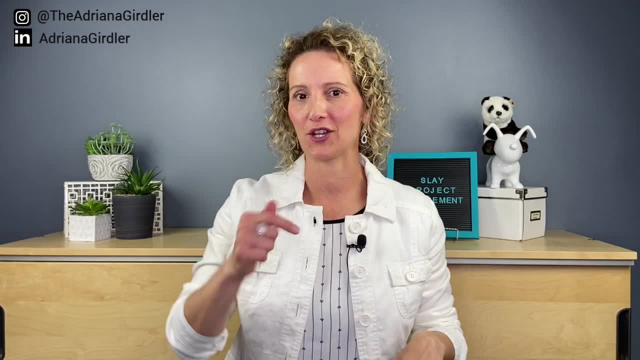 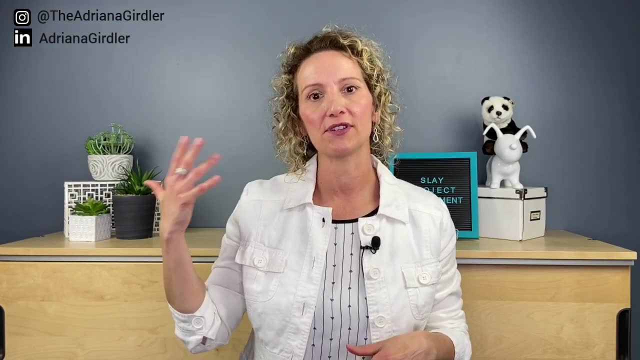 this is an interesting one and tell me if you've ever experienced this in the comments below. But I find sometimes people say: Adrienne, I can't give you timing on projects. I'm like, yes, you can, Particularly when you have senior. 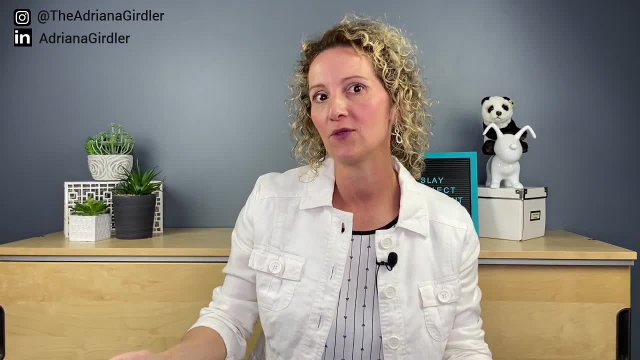 executives who are saying to the project manager: what's the timing of this? When can we expect to get it done? Worse yet, when they have expectations of when it should be done in their eye, but yet that doesn't match up with what's going on in the project. 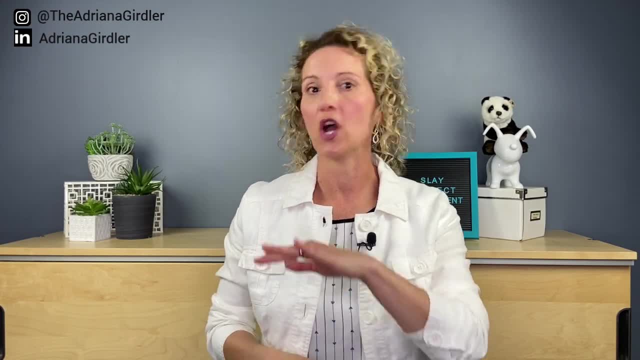 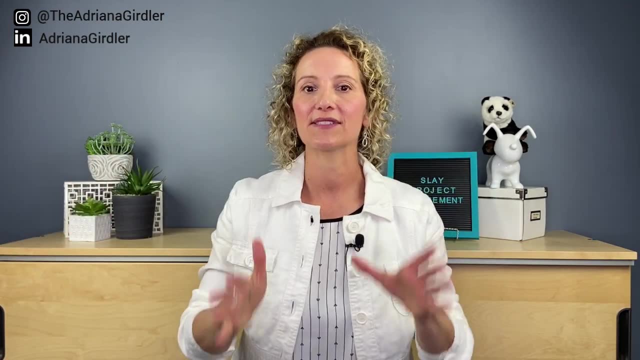 So it's really important at the beginning of the project, not for detailed timing of stuff, because you know what You're gonna get to that much later in the project lifecycle, but you want to at least have some high-level milestone conceptual ideas of timing and that's really important. And at this, 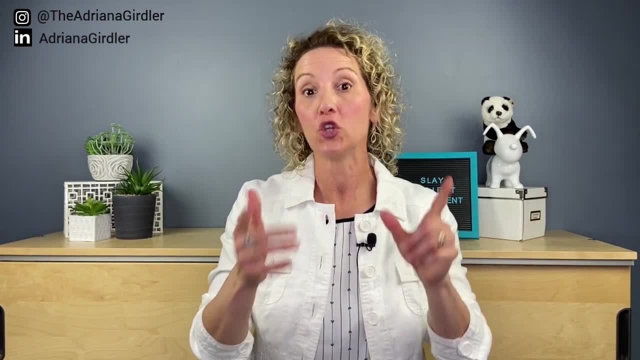 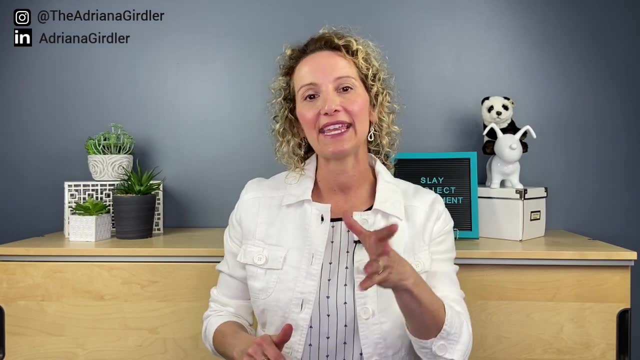 stage with all the information you've collected so far to date, you can do it. You can do things like your go live date. You can then think about all the training you need to have, And the key to doing this is by working backwards. But 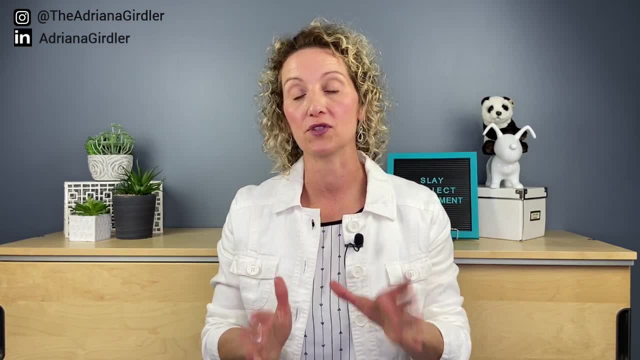 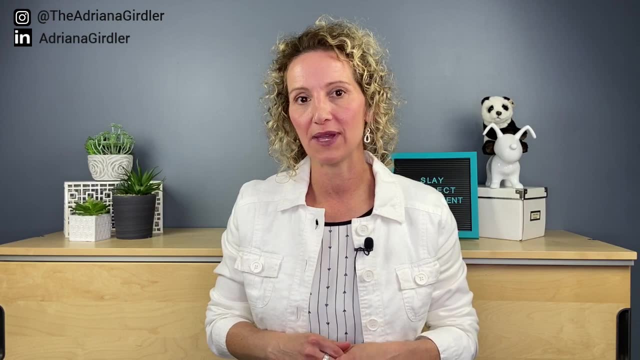 really important that you get a very high-level milestone timing because you know sometimes you have to go back to the sponsors at this stage and say: you know what You want to get this done in six months. I've already did my work back. 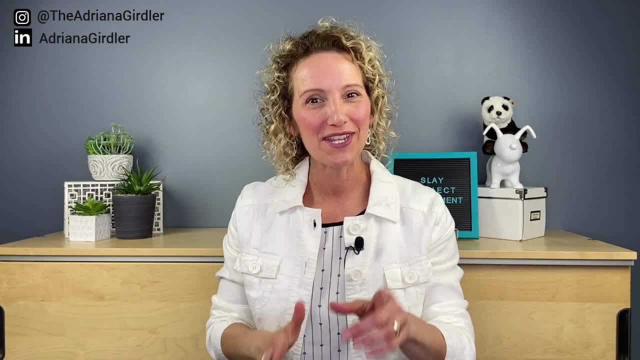 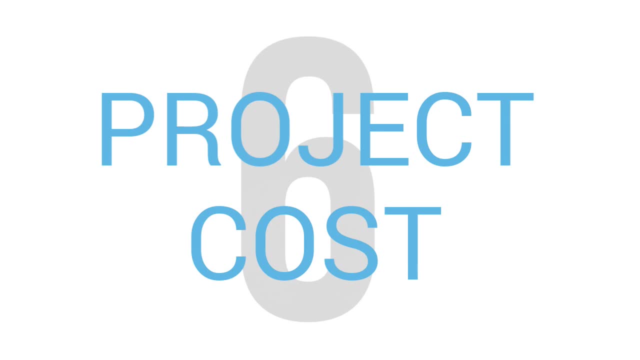 schedule. There's no way it's gonna happen. I need ten And you want to do that negotiation now. That's why this is so important with part of project planning, Step six: project cost. Why did I do that? You know why: Because 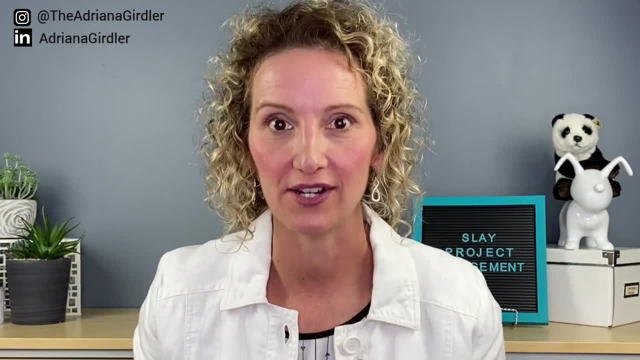 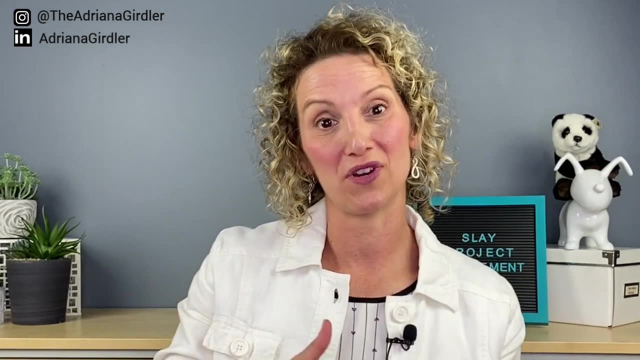 sometimes people think money and project cost is scary. I don't know why. You know what You're running a project. I've never come across a project that was free, because there's direct cost, indirect cost, whole bunch of things associated with it. You're probably gonna have to spend something. 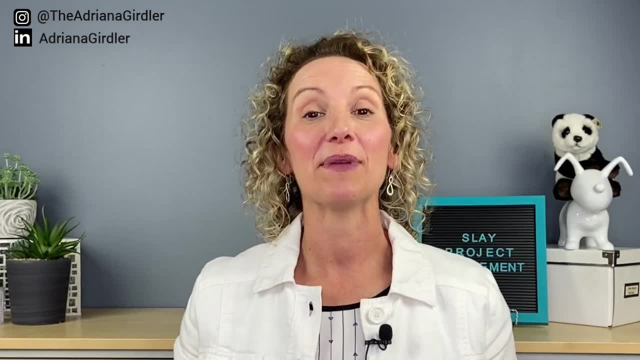 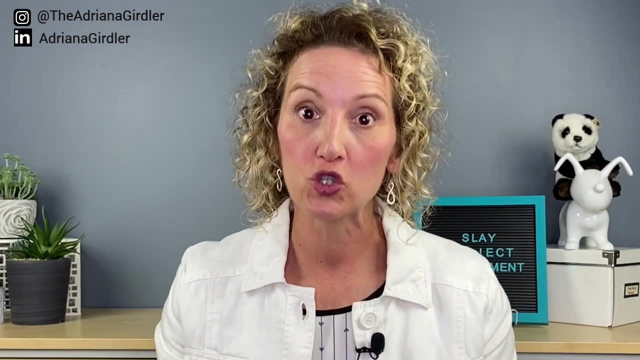 Even if it's just ten bucks, that's okay, But it may not be. It may be a million dollars that you have to spend, But the thing is it's your job as a project lead, a project manager, to look at budget. How much money do you actually have to? 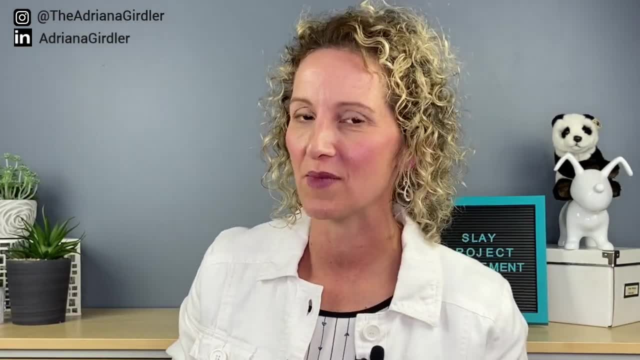 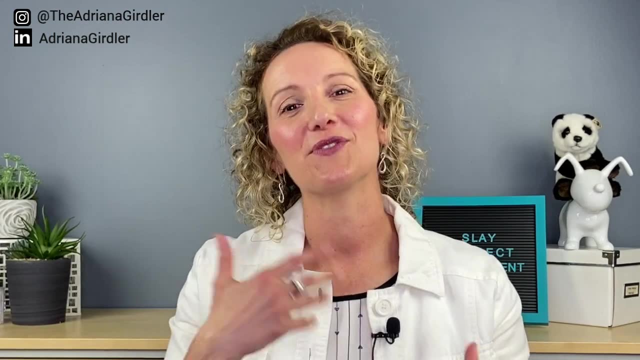 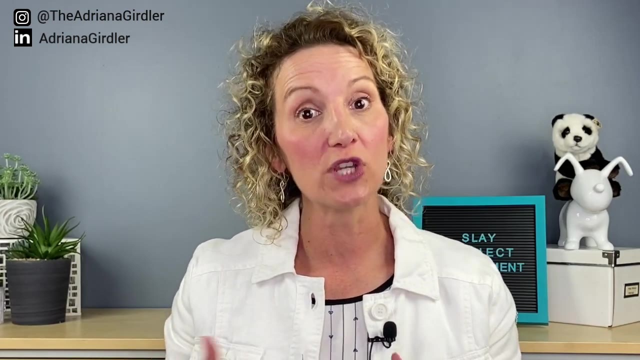 spend. Are there some assumptions made by some senior management that you can execute this project without spending money? Guess what Ain't gonna have happen. So these are the clarity that you need, by asking what is your budget, Because you may have to, in that planning stage, have to re-look at your scope. 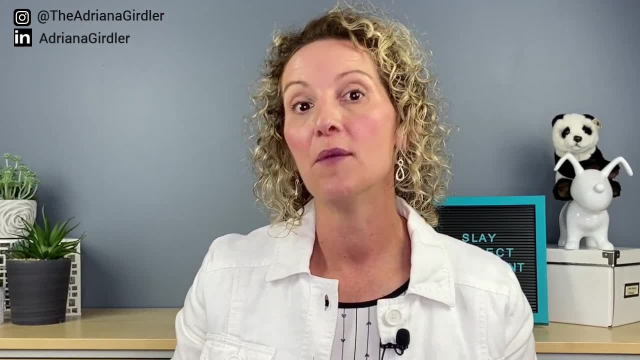 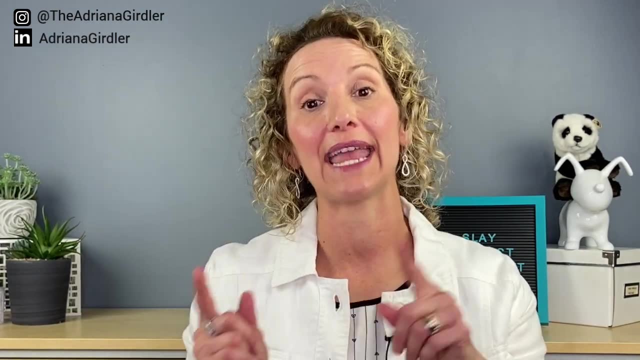 statement And maybe you can or can't deliver on some of those things because you now have a clear idea of what your budget is. So it's really important to ask for what is your budget and plan it in and cross-reference it with the other. 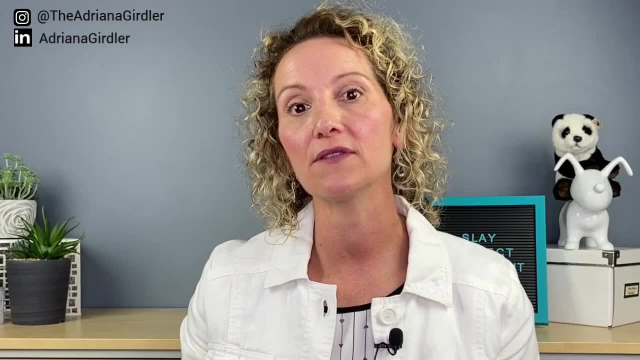 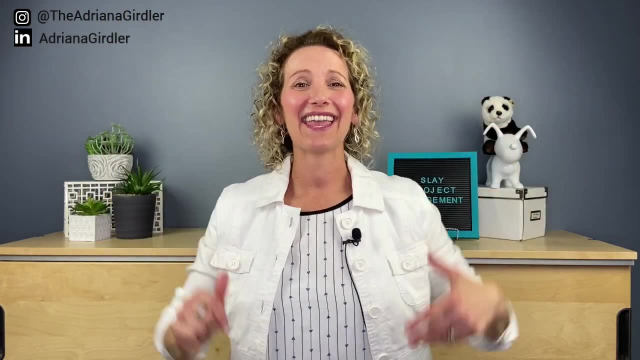 stuff that you have. Can you actually deliver with what you're being asked to deliver with the amount of money that you've been given? Step seven: kick-off meeting: Yay, Now, this is an interesting one, because you notice how it's step. 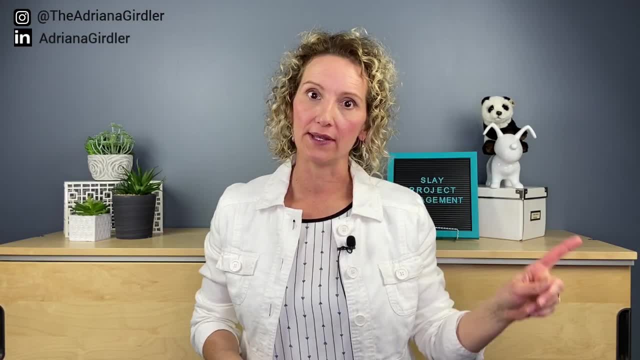 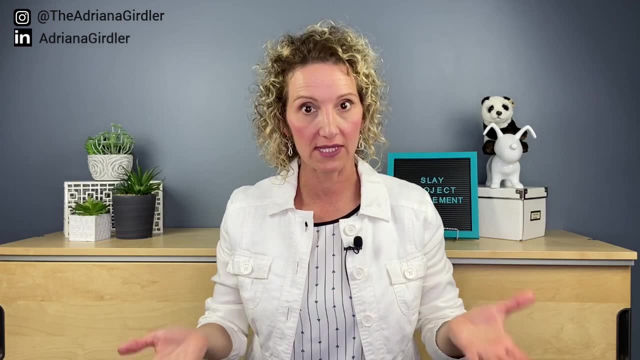 seven kick-off meeting. Some people will make kick-off meeting step one. No, Never, ever, ever, ever do it. Did you see how much work and preparation you had to do before we even got to this step seven of a kick-off meeting? Look, kick-off. 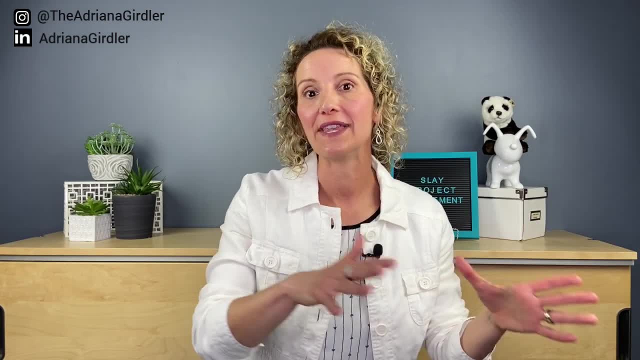 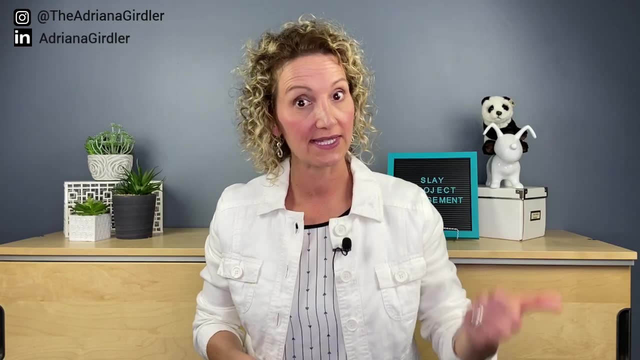 meetings are critical. It's when you bring everyone together with all the necessary information- everything that we just spoke about and that you collected- and you bring your team together because you got that team confirmation and you kick everything off. But you don't kick it off by just telling them there's a project. 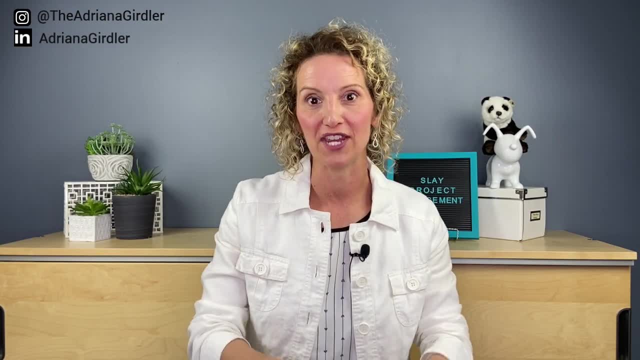 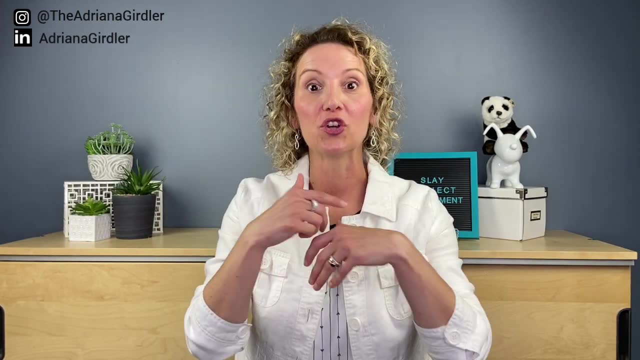 You kick it off by saying: you're on this project. I've already vetted this with your managers and here's a package that I'm giving to you, because we are now at the end of this meeting. you're going to start executing. You're going to start. 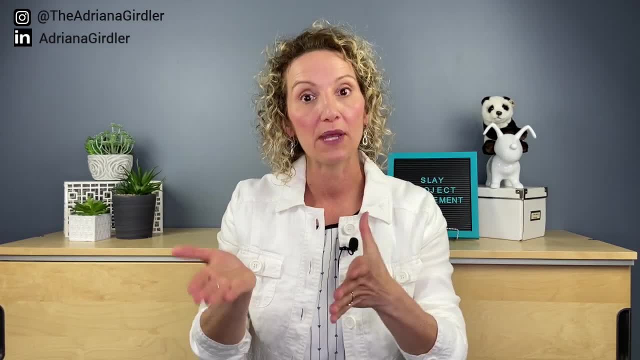 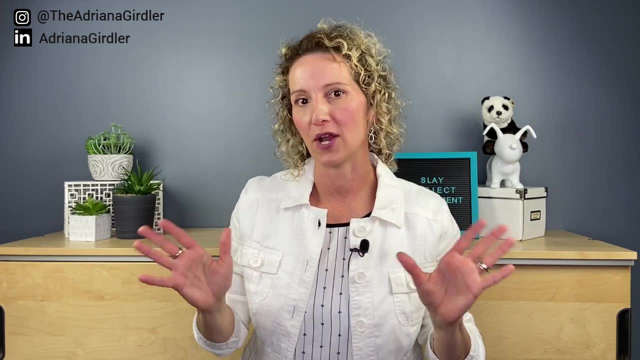 getting into the project and you're going to start establishing those rhythms. That's a part of project planning. So you really have to do all of this legwork. This is why this is a very critical stage in any project. Step eight: this is your project tasks. 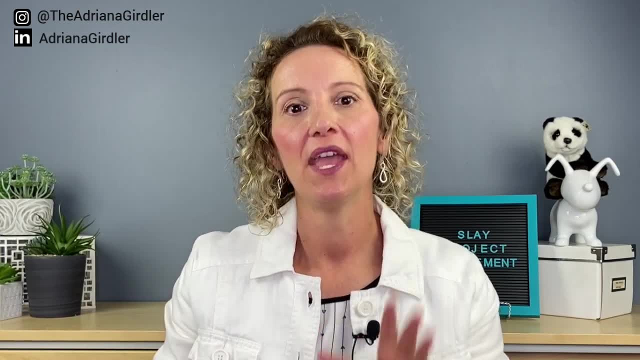 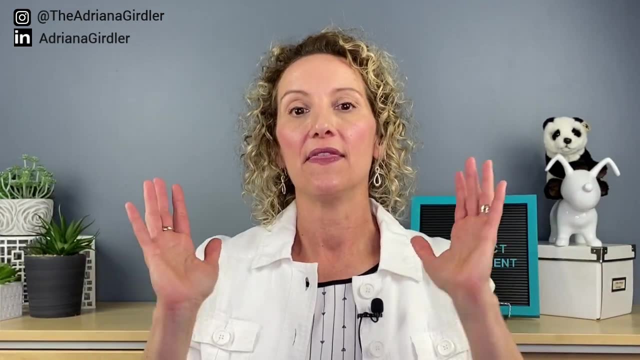 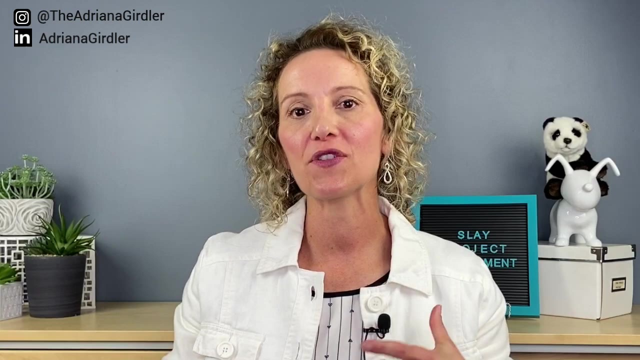 All right. I love this actual part of project management. I find sometimes there's this impression that project managers have to come up with everything and do everything. That is not your job. Your job is to guide and lead a group of subject matter experts and ensure that. 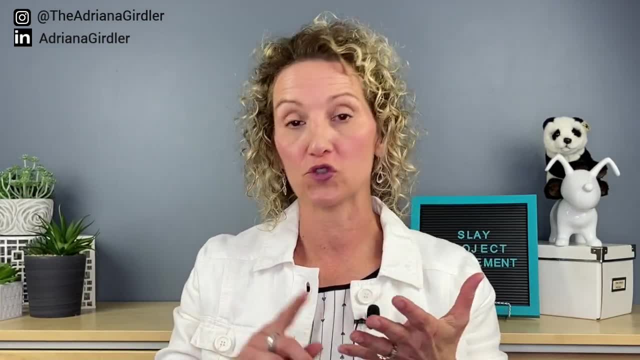 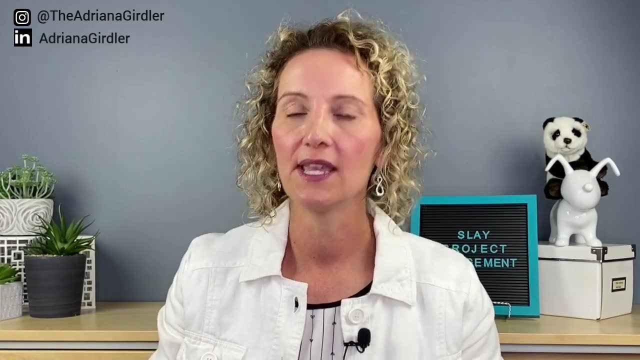 they have everything they need at their fingertips to deliver on scope, time and budget and ensure successful project completion, And so part of that is guiding them with tasks. So you want to be creating with your team after your kickoff, based on all the information you gave to them. 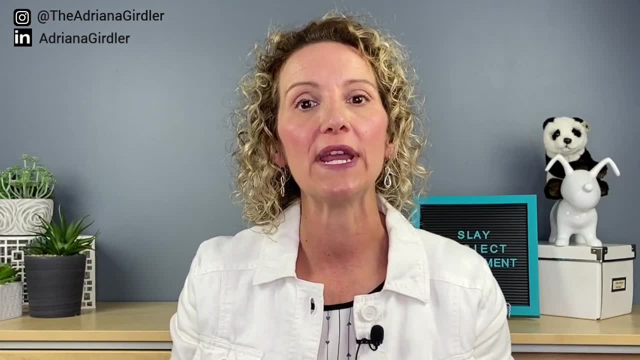 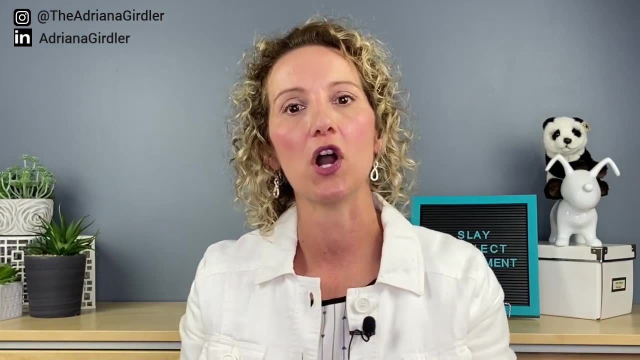 and particularly with their subject matter expertise. what is it we need to do to be successful? Break them off. Have them do it in pairs and groups that make sense to what they're going to be working on together. Now, why do I do this? 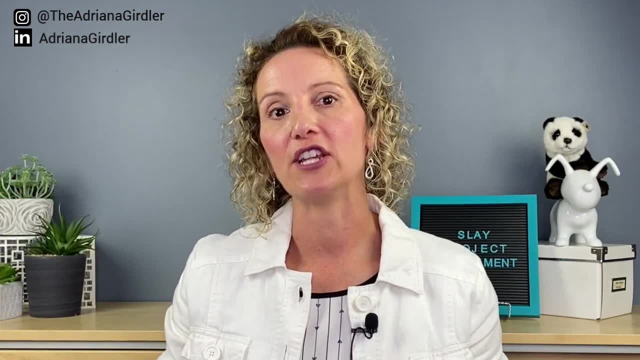 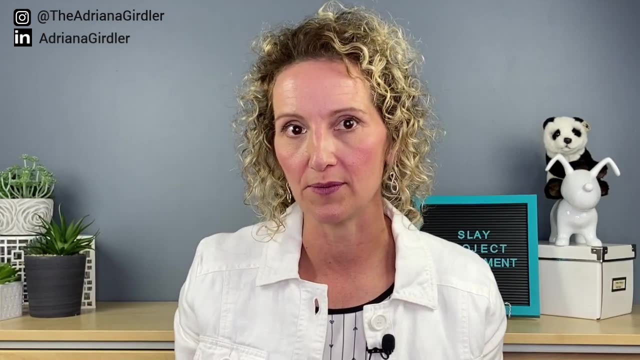 It brings accountability. That is huge. I find too many times some project managers are chasing their project team members. Why? Because the team member doesn't feel accountable. But if I'm a subject matter expert and I'm telling you, oh, we have to deliver on this ABC. 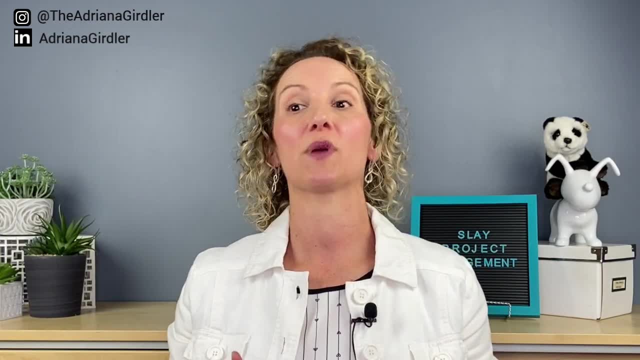 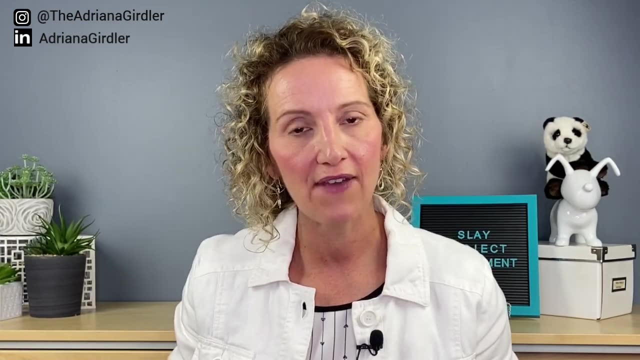 and I know, as a subject matter expert, who's going to be implementing this and who's probably going to be in the heart of it. I need to do X, Y, Z, then you know what Great. You tell me how you think that's going to have happen, And it's my job to collect all of that information. 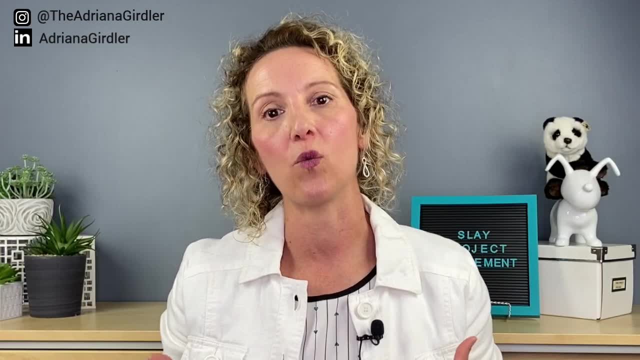 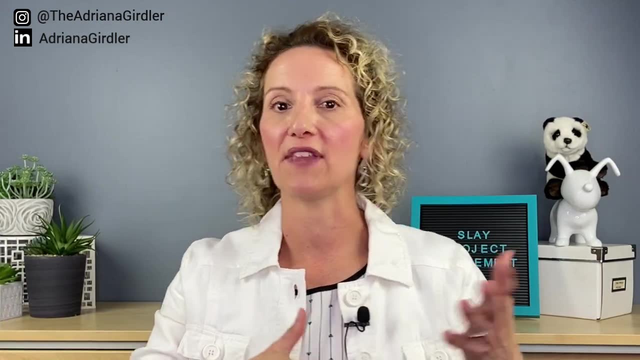 and put it in some sort of sequencing and flow to make sure that we can address it. Yeah, Down the road you bring in agility, You have the ability to work on things and have some flow and change things up, But you really do need at your first kick. 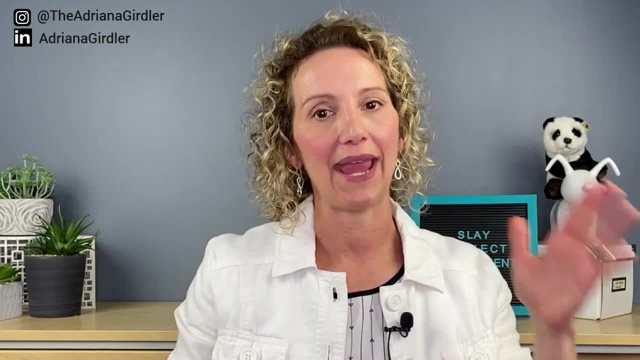 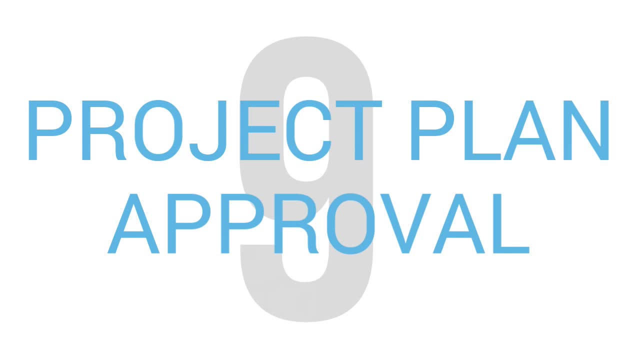 what is all the high-level stuff we all need to work on, from A to Z, to make sure that this is successful. Step nine: project plan approval. What, Adriana? we just had a kickoff. We did it. I just want everyone to go: Whoa, whoa, whoa, whoa, whoa, whoa, whoa. 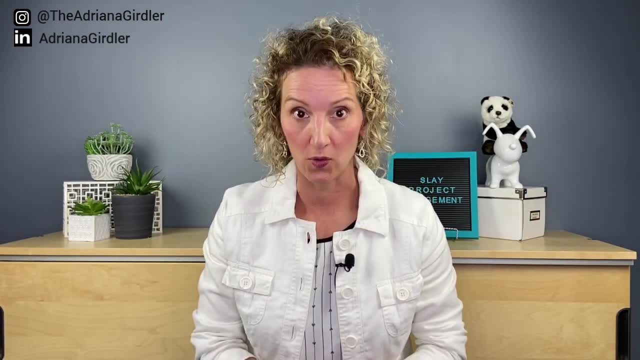 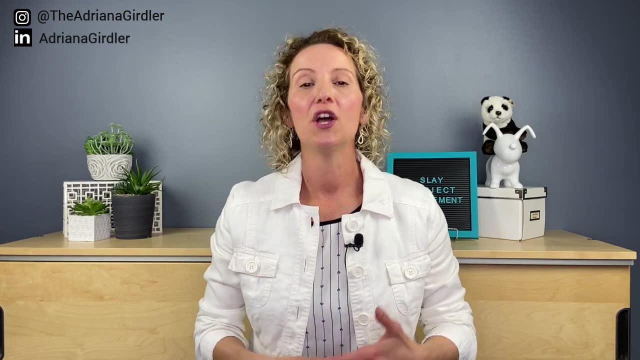 Unfortunately, projects are done within organization. There is hierarchy within organizations. Not only that, you have a sponsor and senior executives who are on your steering committee who need to be aware of what's going on. There is a little bit of channel a channel. 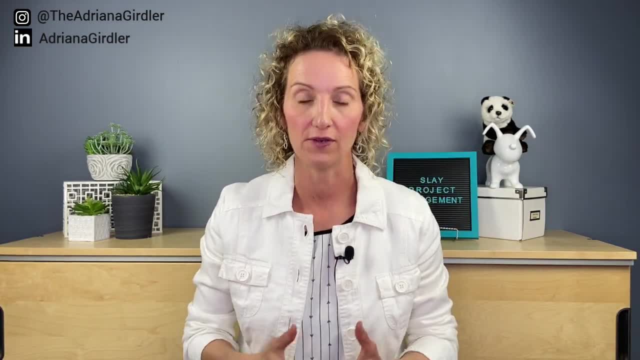 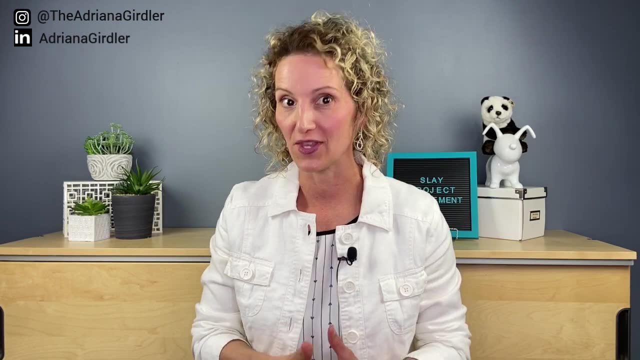 of command, a hierarchy of command that you do have to follow. So once you've created everything with your team, then you do want to present that back to those who are decision makers, really the ones that approve the decision. Then you have an agency. Those are the agencies that approve budgets and are going to ensure that. 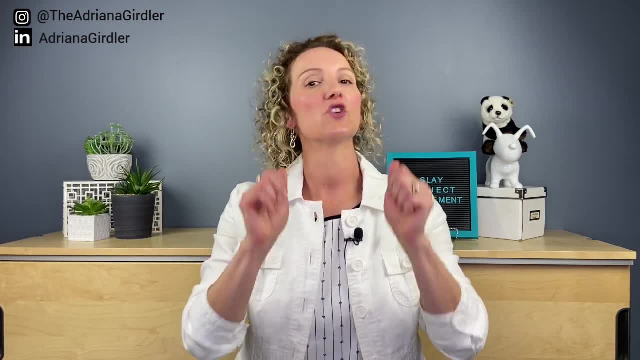 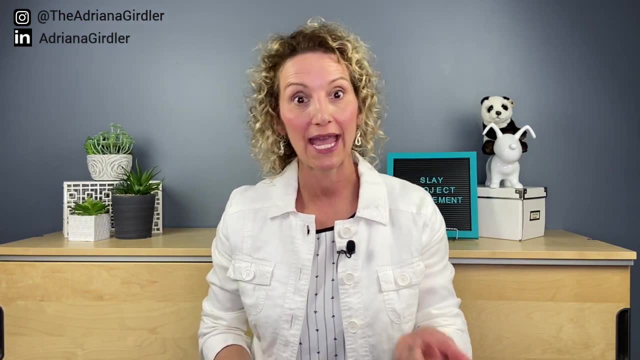 your team members can be successful because they can remove roadblocks. So you want to go to them saying, hey, do you approve what our plan is? They may have had some assumptions and perhaps you did do your due diligence and tried to capture them, but now that 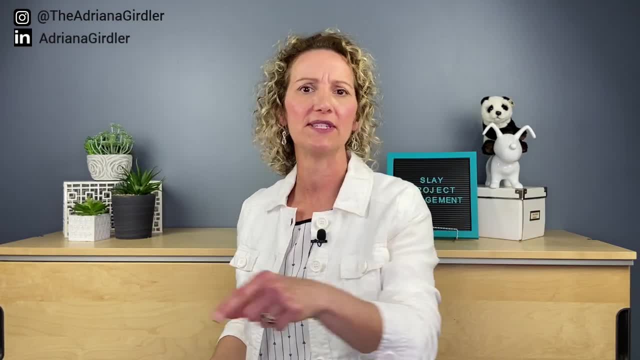 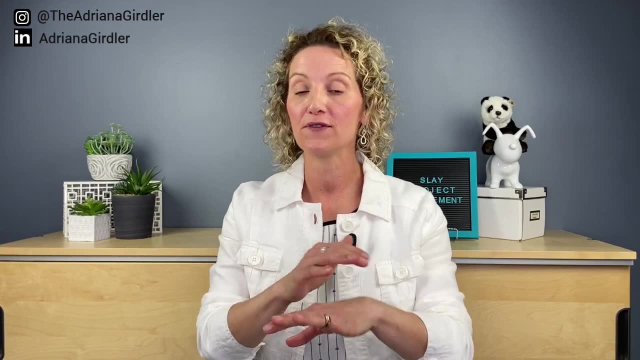 you brought the plan to them, they're like: whoa, what about this? I thought this was going to be done earlier. You can do lots of negotiation at this point and you really do want to have that approved first kick of the can. Step 10, project plan execution. Whoa, I'm going to get my name out there. I'm going to go to my writing room, which is right in the middle of this room- the marketing stuff. I'm going to go to my website, my analytics, and then I'm going to go to my 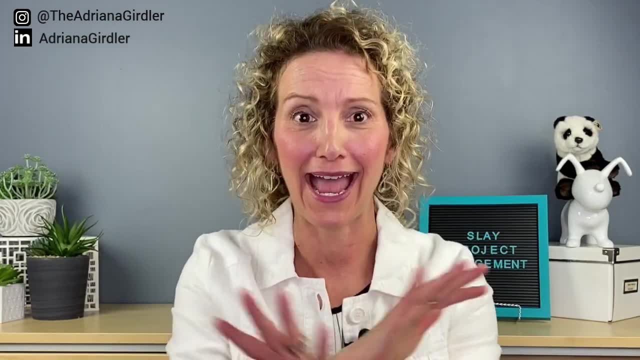 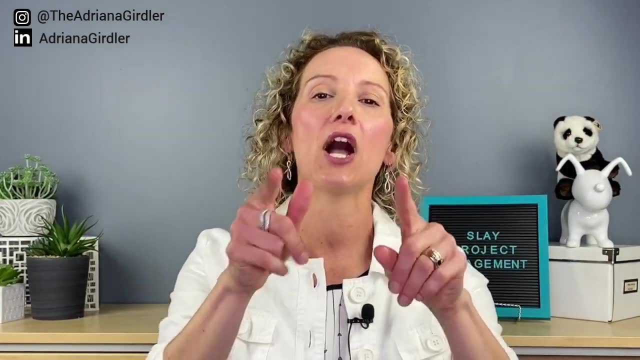 Oh my gosh, you did it. You created a project plan, And how cool is that? And you've done it in the right sequencing event, You've gotten the right people involved, You've got all the approvals. It is time for you to now start executing. And how great is it that you can.